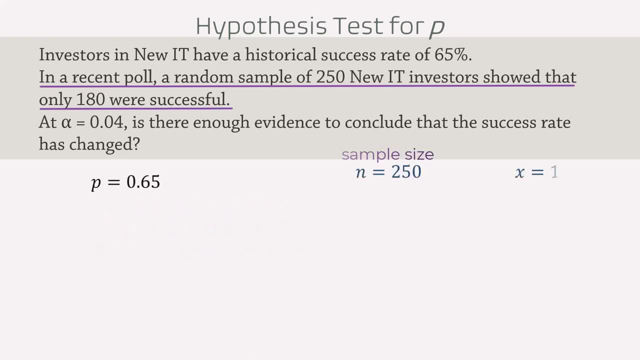 That means we have a sample size n of 250 and the number of successes x of 180.. The sample proportion p hat will thus be 180 over 250, which gives 0.72.. At alpha equals 0.04, we want to test if there is. 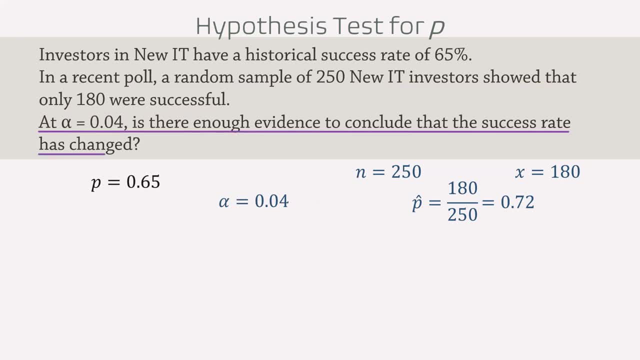 enough evidence to conclude that the success rate has changed, that it is chained or different from 65%. Therefore, the alternative hypothesis will be p not equal to 0.65.. And the null hypothesis is p equals 0.65.. Next we can calculate the test statistic by substituting the values: 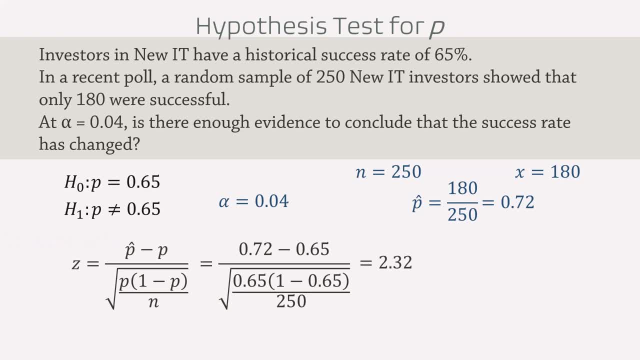 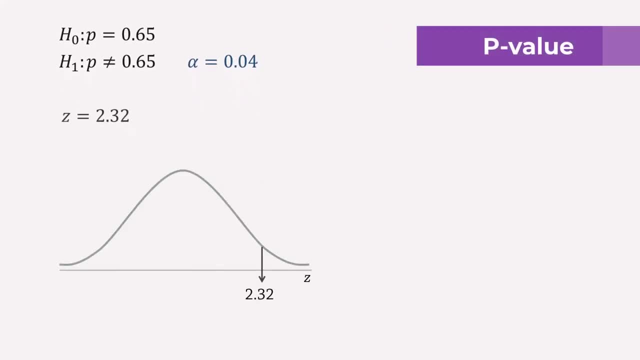 into the formula, And that gives 2.32.. Now then, we can calculate the p-value of this test by finding the area in detail beyond this test statistic. under the normal curve, The p-value is the probability of finding a sample statistic as extreme as we obtained, given the null hypothesis is true. 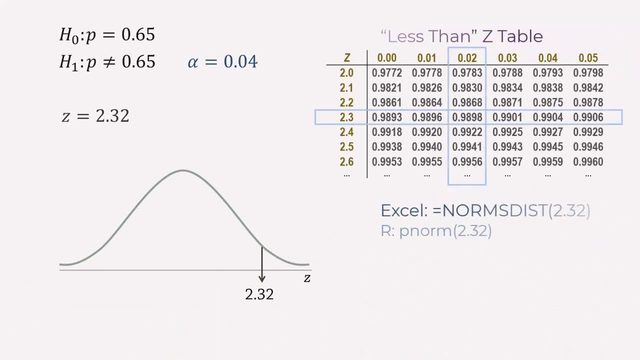 Using the less than normal probability table, the area corresponding to 2.3 under 0.02 is 0.9898.. The upper tail area is thus 1 minus 0.9898, which gives 0.0102.. Now, since this is a two-tailed test, 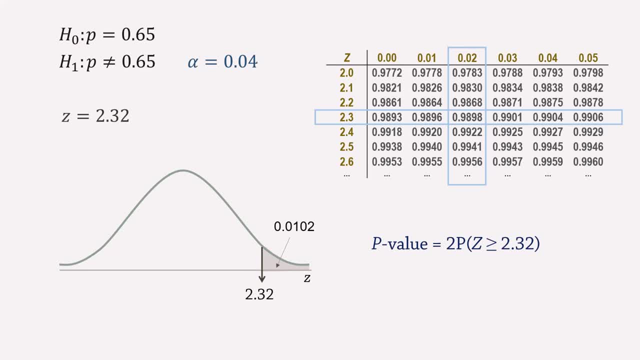 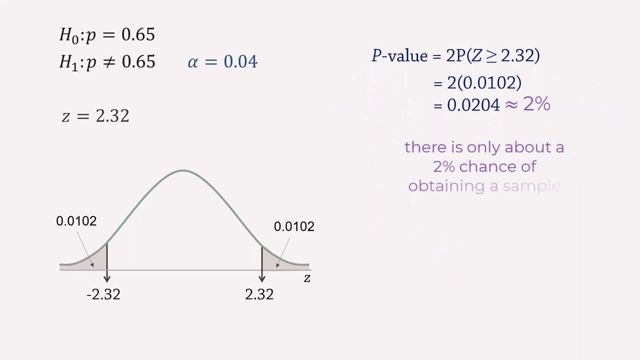 we can calculate the p-value of the sample result. The p-value is obtained by multiplying the one-tailed area by two, that is, adding the corresponding lower tail area. Therefore, we have a p-value of 0.0204.. So what does this tell us? It tells us that there is only about 2% chance of obtaining 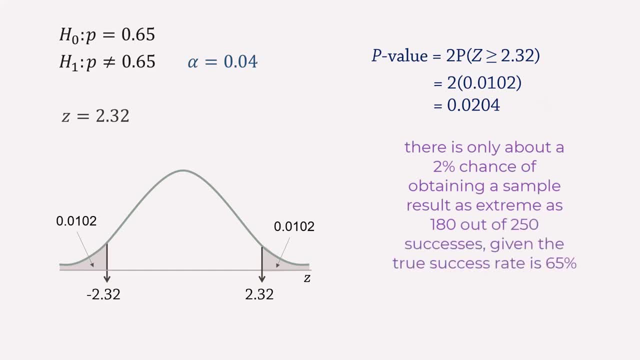 a sample result as extreme as 180 out of 250 successes, given the true success rate is 65%. Now let's look at the null hypothesis if the calculated p-value is less than the significance level alpha. Since this p-value is less than an alpha of 0.04, we will reject the null hypothesis. 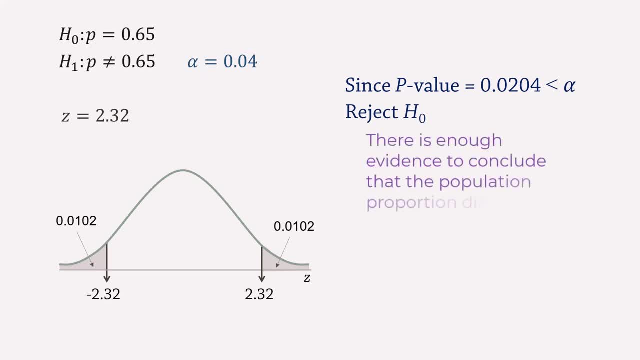 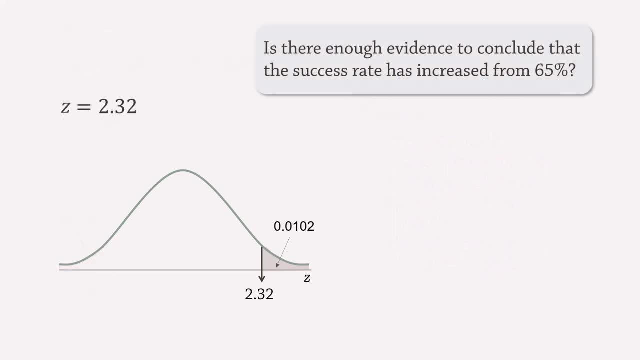 and we have enough evidence to conclude that the population proportion now differs from 0.65, or that the success rate has changed. Now suppose instead we want to test if the success rate has increased from 65%, Then the alternative hypothesis becomes p greater than 0.65. 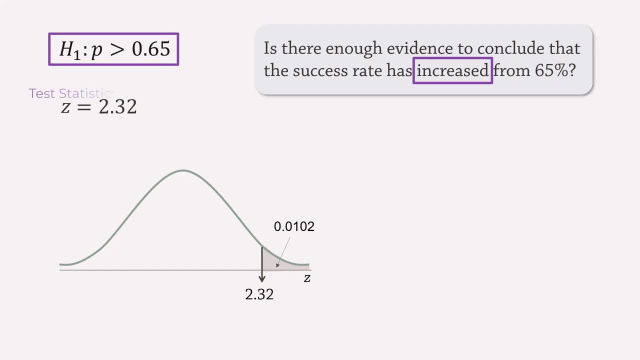 Greater because of the keyword increased. The test statistic will not change, but we now have a one-tailed test, In particular a right or upper tailed test, And thus the p-value will be the area to the right of the test statistic, which is 0.0102.. Now, if alpha equals 0.04, we will again. 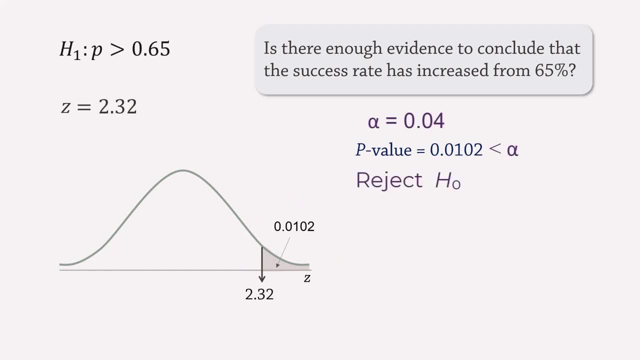 reject the null hypothesis, since this p-value is less than alpha and we will conclude that the success rate has increased. But if alpha were 0.01, we will fail to reject the null hypothesis, Since this p-value will be greater than alpha. that is, at alpha equals 0.01,. 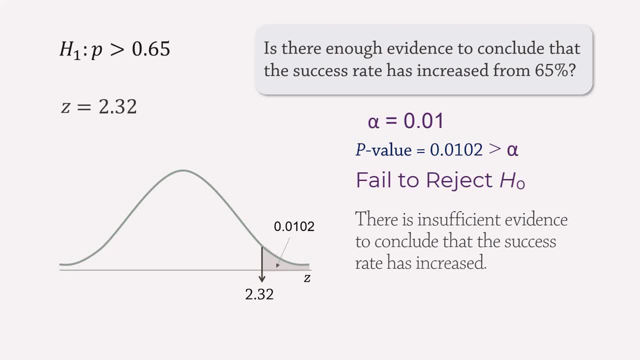 there is not enough evidence to conclude that the true proportion is greater than 0.65.. Now suppose we were to test if the success rate has significantly decreased from historical values. Then the alternative hypothesis will be p less than 0.65 because of the keyword decreased. 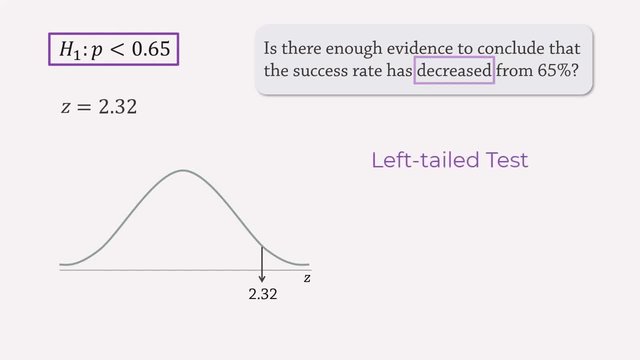 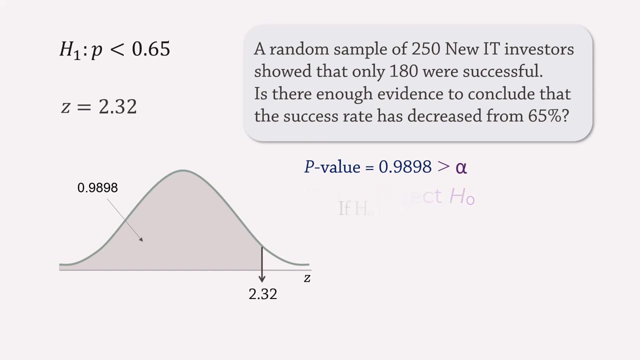 This will be a left-tailed test. Therefore the p-value will be the area to the left of the table, the test statistic, which is 0.9898.. This p-value is much larger than our conventional alpha levels, so the null hypothesis will not be rejected. It means, if the null hypothesis is true, that is. 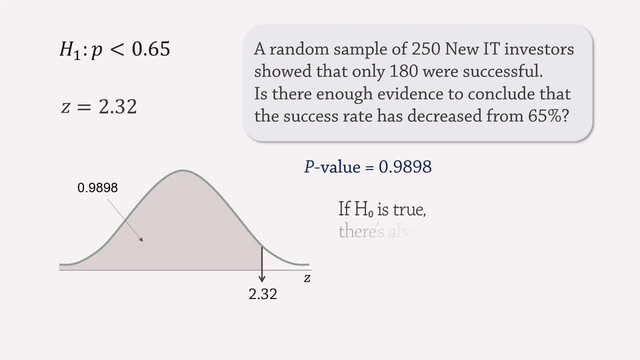 the success rate is indeed 65%, then there is about 99% chance that we will find less than 180 successes in a sample of 250 investors. Note, however, that the typical left-tail test results more often in a negative test statistic. Otherwise, a hypothesis test may. 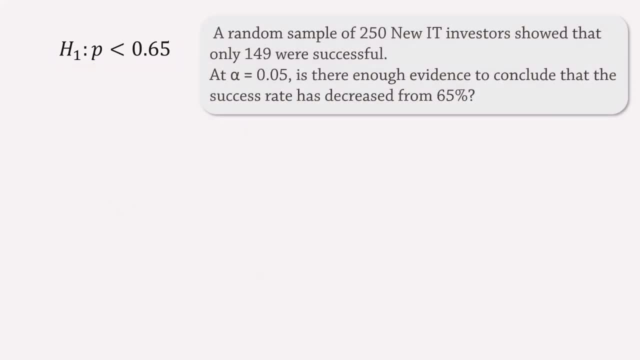 not be necessary. A typical left-tail test example could be the case with 149 successes out of 250, and we want to test if the success rate has decreased from 65%. The sample proportion is now 0.596.. Plugging in the values, the test statistic is negative 1.79, and the less-than area is found. 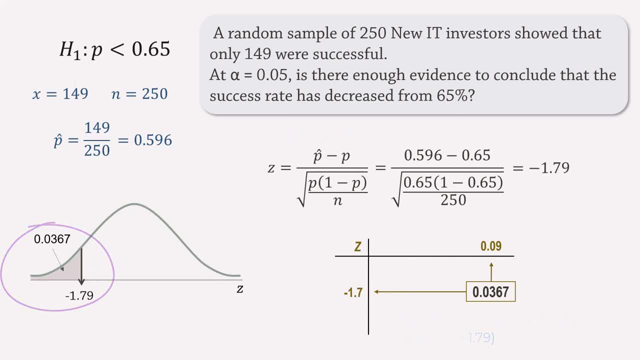 to be 0.03.. The test statistic is negative- 1.79, and the less-than area is found to be 0.03.. Since this is a left-tail test, the p-value is 0.0367,, which is less than the specified alpha of.